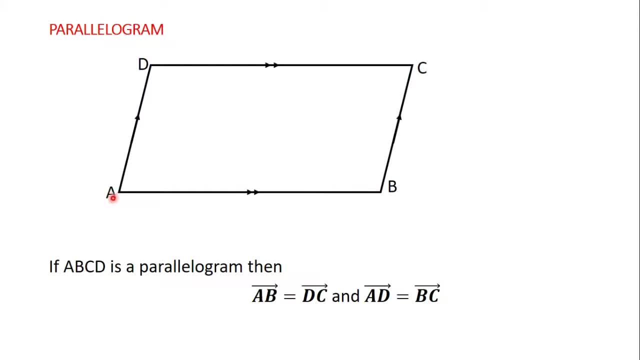 diagram ABCD. you can see that line a- b is a vector, so it's indicated here with the arrow, and line d- c is also a vector. ad is a vector and b c is also a vector. ad is a vector and b c is also a vector and b c is also a vector. 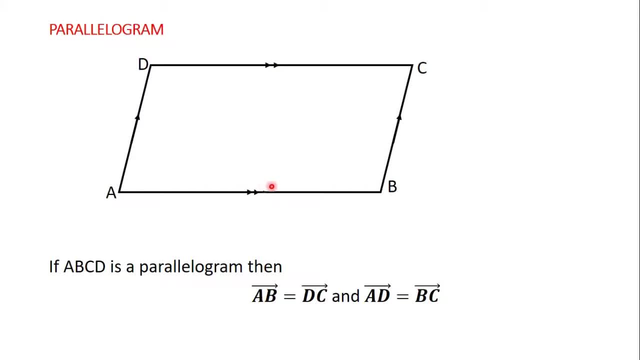 a vector. if this is a pyrogram, then the vector AB is equal to the vector CD and the vector AD is equal to the vector BC. this is a special property of a pyrogram. so if you have a pyrogram like this, vector AB is equal to vector BC. 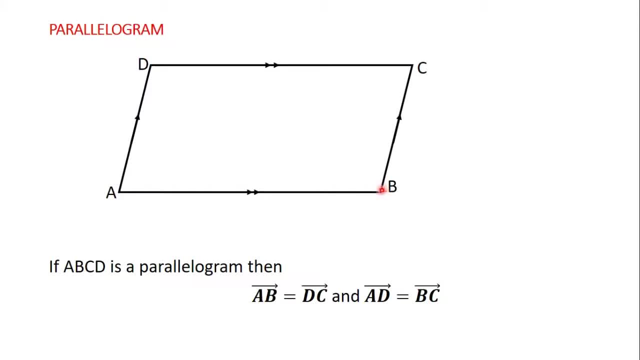 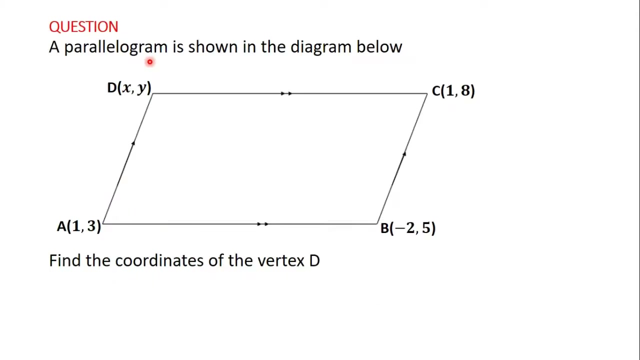 then vector AD is equal to vector BC. that is what you can see here. so vector AB is equal to vector DC and vector AD is equal to vector BC. with this property, we can find the coordinates of one of the vertices. let's pick some, let's pick a question and see how to do this. so a pyrogram is shown in the. 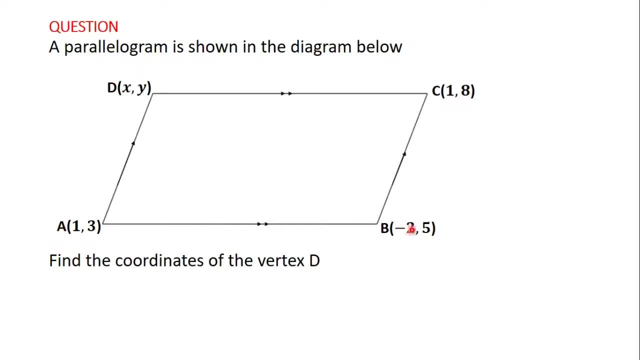 diagram below. so we have this pyrogram here: ABCD. okay, find the vertices of D. so you see that the vertices D have the coordinates XY, so you have to find the vertices. what that means is that we need to find X and Y. we have the vertices A to be 1, 3, the vertices B as negative: 2, 5. 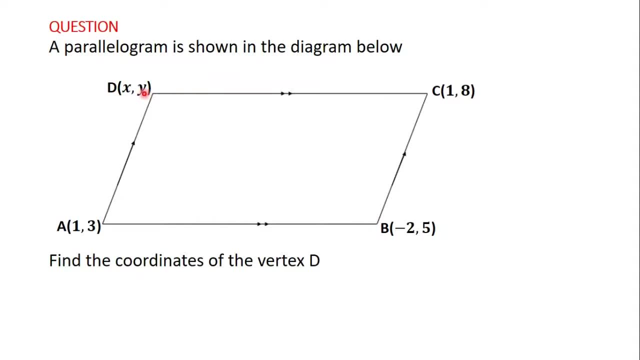 vertices C is 1- 8 and the vertices D is XY. how do we find the vertices D? we know that if this is a pyrogram, then vector AD is equal to vector BC. someone can also say: vector AB is equal to vector DC is the same thing I'm using. 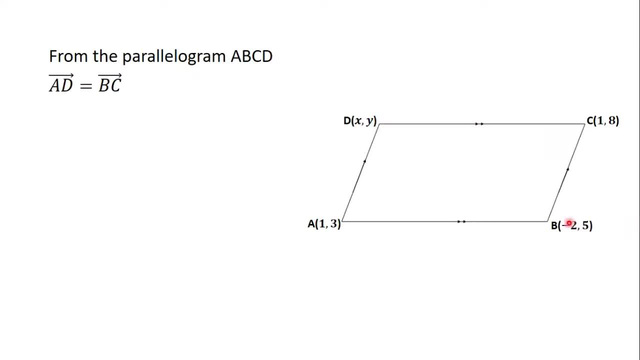 this one. so vector AD is equal to vector BC. but what do we know about vector AD? we know that vector AD is the same as position vector D minus position vector a. we've learned this in the previous video. so vector ad is equal to od vector od minus vector oa, which is the same as position vector d minus position vector a. 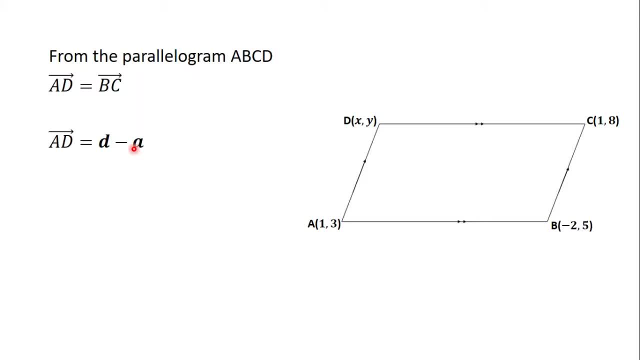 i'm sure that by this time you are conversant with this. that is why i did not write the od and oa. so here, when i write small letter d, you know what i'm talking about. when i write small letter a, you know what i'm talking about because we solved a lot of examples okay, so the vector ad is the same. 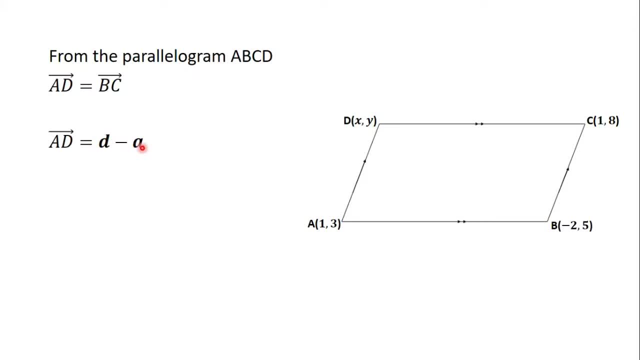 as position vector d minus position vector a. what are the components of position vector d? the components of position vector d are the coordinates of the of the point d. the coordinates of point d are x and y, so the components of position vector d are x, y, minus the components of. 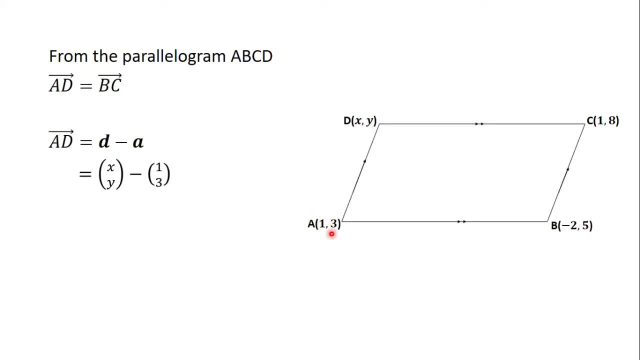 position vector d are x and y, minus. the components of position vector d are x and y. vector a are the coordinates of point a. the coordinates of point a are one and three or one three, so the components of position vector a will be one three. we know that from subtraction of. 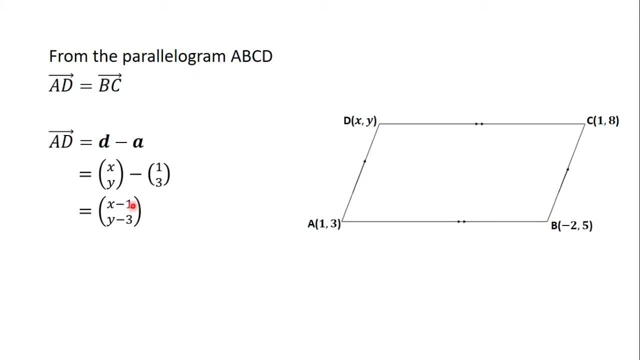 vectors x minus one will give us x minus one, then y minus three will give us y minus three. so we have been able to find the first part here, which is ad. let's move on to the second part. bc position vector bc will give us position vector c or oc minus position vector b or ob. so ob oc is. 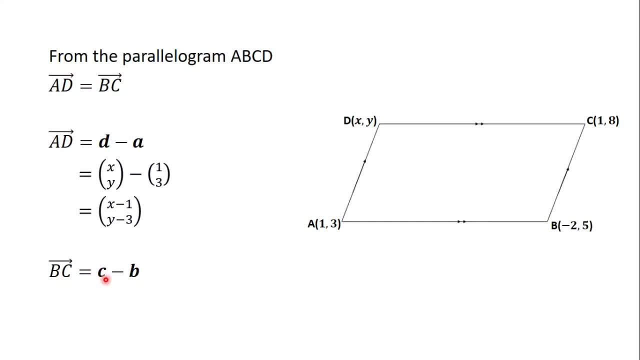 the same as position vector c or small letter c. as you can see here, then, ob is the same as position vector b or small letter b. the components of c here will be the coordinates of point c, which are one eight. so the components are one and eight. 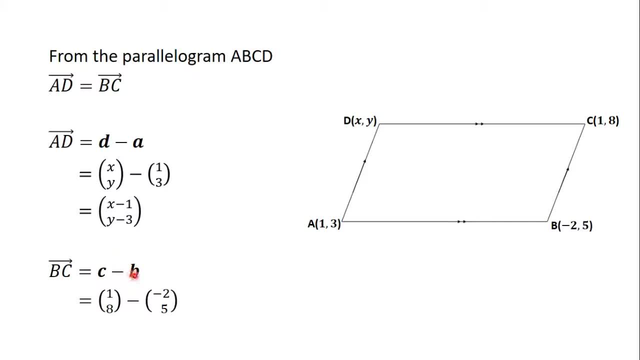 now minus the components of b. here will be the coordinates of b, which are minus two, five. so if you do the subtraction, you have one minus minus two, which is three, then eight minus five, which is also three. so look at something here we have been able to find.